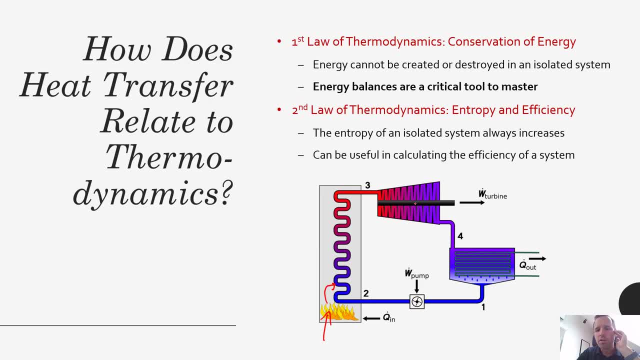 That steam would be used to create power. There'd be another heat transfer process here, where you are removing heat, And then this cycle continues, This process. you don't just take fuel and convert 100% of that into useful work. You're going to be losing energy along the way, which is how the second law of thermodynamics comes in. 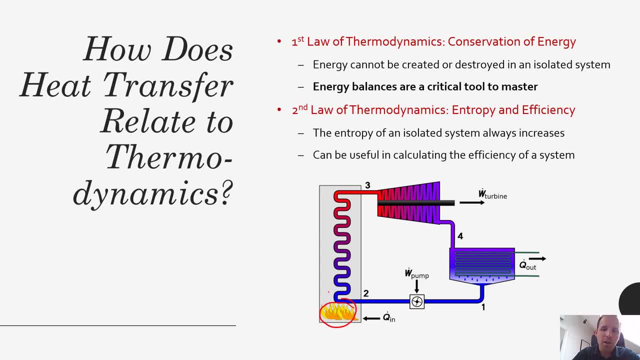 So naturally you're going to be burning a fuel here, but you can't get 100% of that heat into your steam. Some of it's going to be lost because entropy is being generated. You're not able to, And then some of it's going to be lost because you have 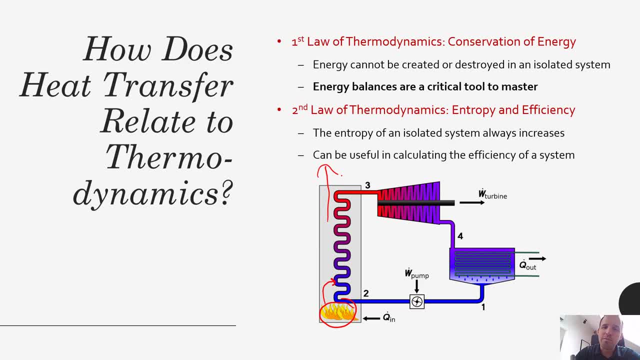 the effluent and this hot gas is leaving your system. So there are definitely some really useful relationships between thermodynamics and heat transfer. And I do want to point out this graphic is not from our textbook, So the definitions here don't exactly match up to the ones that I laid out in the last lecture. 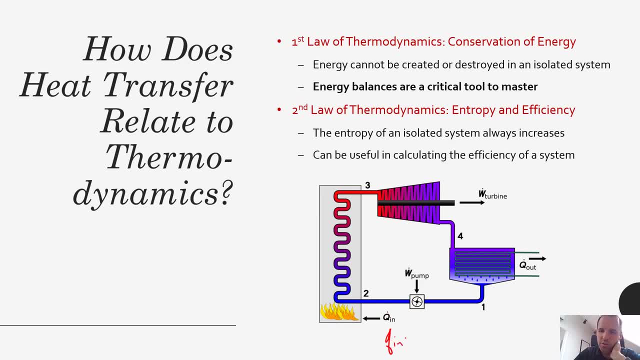 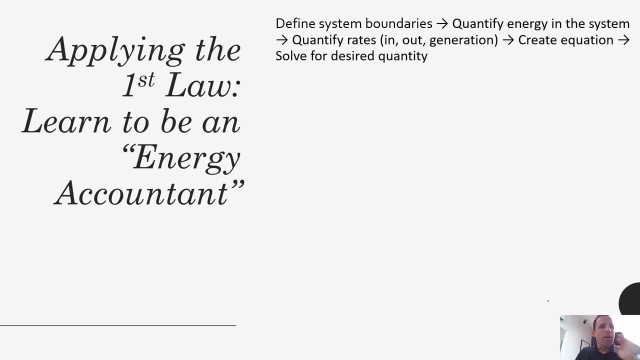 We'd actually use little q in here to represent a rate of heat transfer, And here we'd use little q out with no dot. Okay, so when you're doing energy balances to solve heat transfer problems, I want each of you to learn how to be an energy accountant. 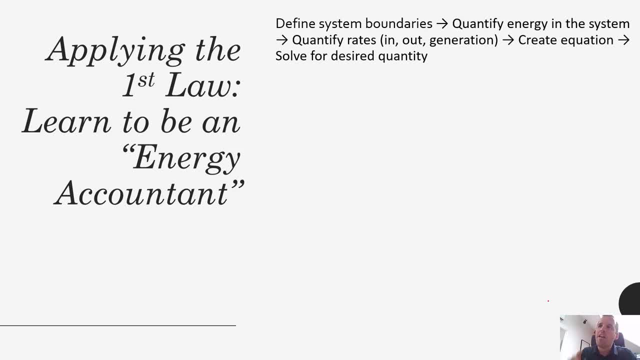 So what does an accountant do? They keep track of how much money are in certain accounts, how much is coming in, how much is going out, how much might be generated from something like interest, or lost from something like a decline in your pay, interest or something. 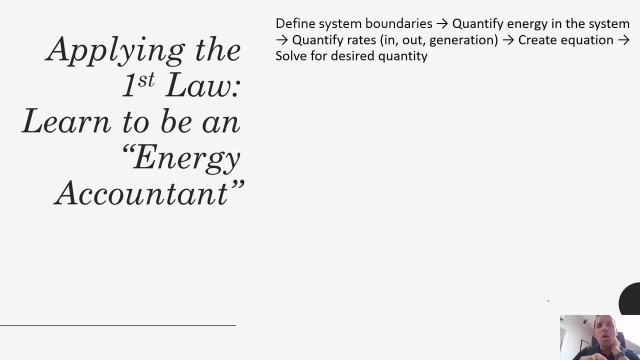 So we'll follow these simple steps. So first we're going to define our system boundaries. So what? how much material is in our system? over what lines is it crossing when it's going in or out of our system? We're going to quantify, okay, how much, if I've defined these boundaries. 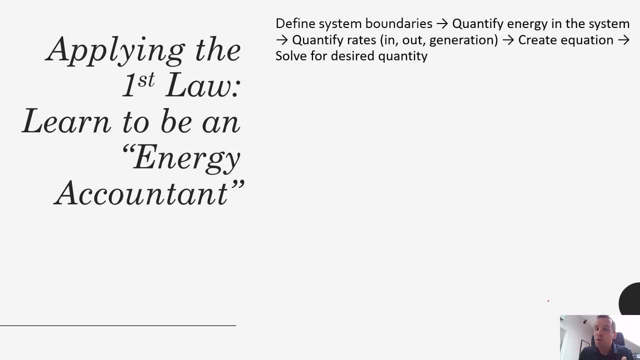 how much energy is in the system at a given time. That will be our accumulation term. We'll learn to quantify rates. This is where the three rate laws of heat transfer are going to come into play. We're going to define these in and out terms. 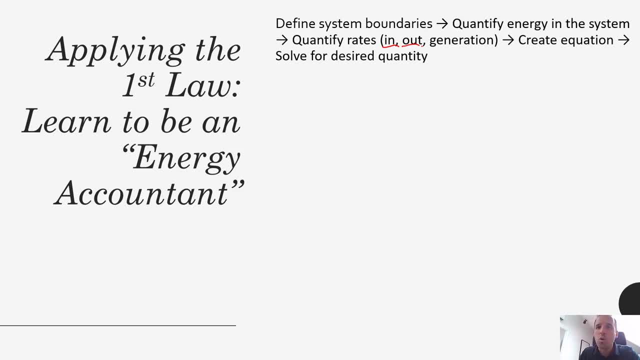 which will always be by either conduction, convection or radiation, or by some some combination of those three. Our system can also generate thermal energy, So that'll be another term, Or it could. it could also be consumption. I just used generation, because consumption could be just a negative generation. 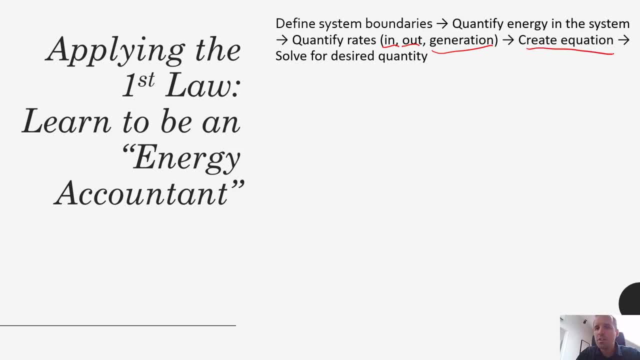 Once we have quantified all of our rates, that'll give us a nice equation and we can take that equation and use that to solve for the desired quantity. So it's really important to be able to carefully account for all terms. You, if you, do this, 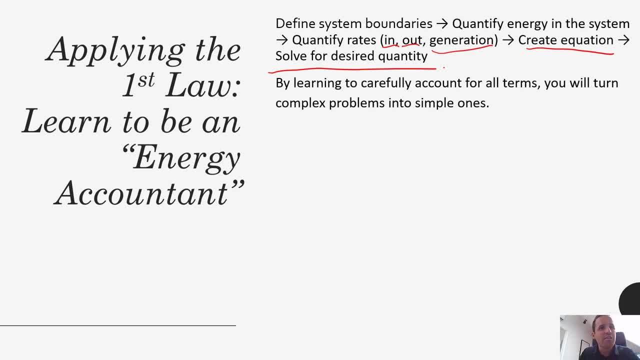 if you're very carefully accounting for all these things, it'll take very complex problems and turn them into very simple ones. So it's very important to create this system and to get into this mentality of how do I be very systematic about doing this. 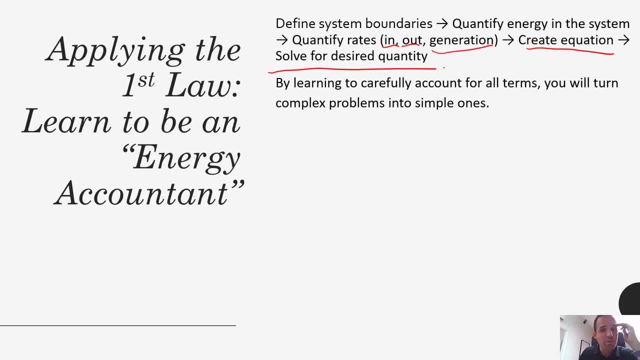 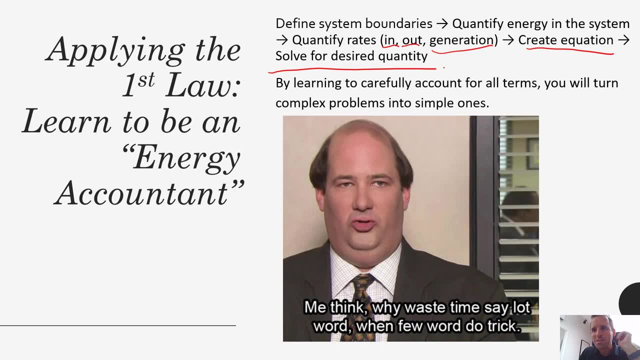 So accounting could be really simple if you're starting to do use these systems. And just as an example, I'm going to show the world's favorite accountant, Kevin Malone, from The Office. This is one of his systems And this is me think. 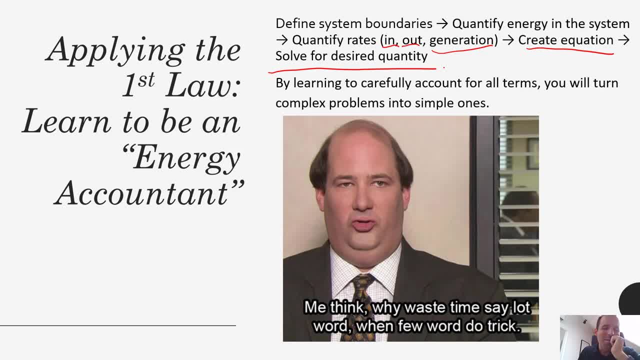 why waste time to say lot word when few word do trick? So I put this in here to be facetious, but also to point out: if you can really simplify problems, you can make them easy, so that even someone like Kevin Malone could solve these problems. 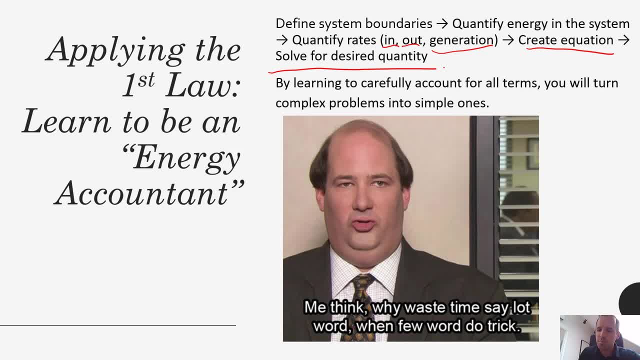 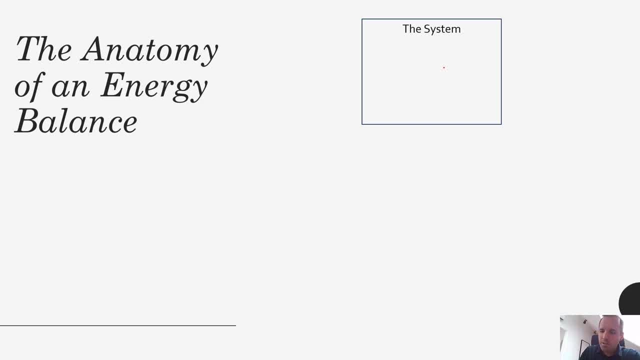 But also we're going to really work hard to develop systems to really simplify these problems that we're going to be solving. So if we take some piece of matter, we'll call that our system. Let's say this is a part of a wall. 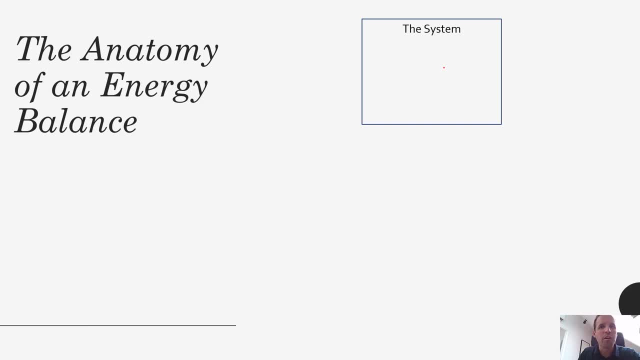 or it could be a block of air in a room, or it could be a big chunk of solid earth. It could be just about any different type of physical space. The first thing to do is decide: okay, what is my system? Is it the air inside of a room? 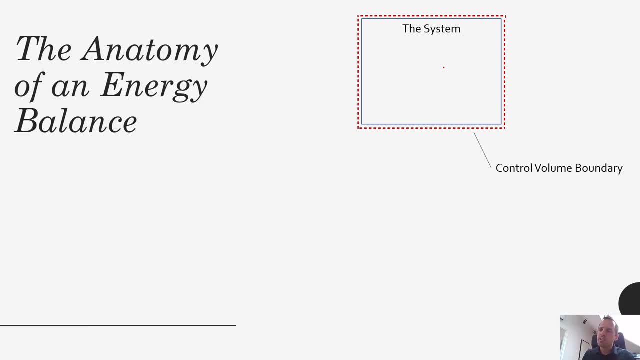 or is it the air inside of a room plus the walls, Or is it the entire house, Or is it the entire neighborhood? So energy will be conserved in that control volume boundary, no matter how you define that control volume boundary, except you're going to want to learn to define control volume boundaries. 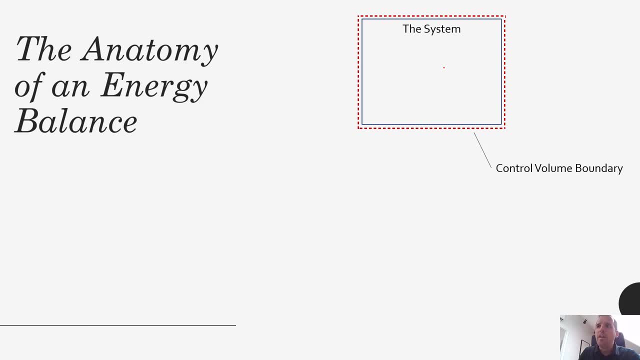 that will create an equation that will eventually be useful to you. So, if you're trying to figure out the temperature inside of an individual room in a house, having an energy balance over an entire neighborhood probably won't be all that useful to you. However, if you're trying to maybe figure out 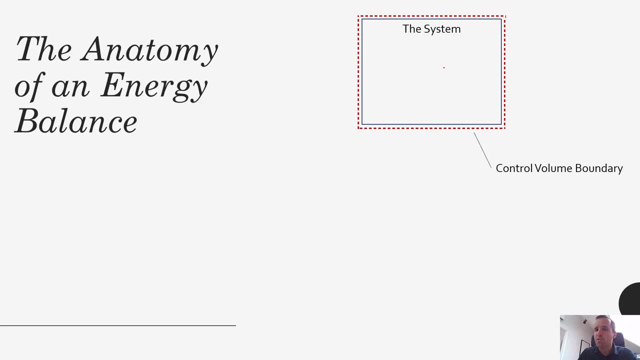 the total energy consumption of your whole neighborhood, then naturally, yes, you'd want your entire neighborhood to be the system boundary. So an energy in term, this Qn, would be energy that's flowing across that boundary into our system. There could be multiple terms. 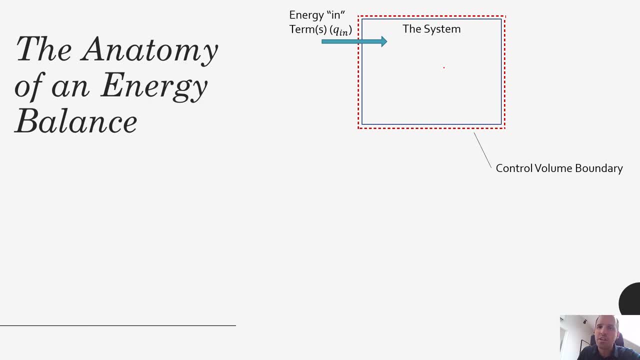 There could be multiple different sources of energy coming in. Similarly, we're going to have energy going out, So this could be going out by conduction, by convection, by radiation or any combination of those three. We could also have generation. 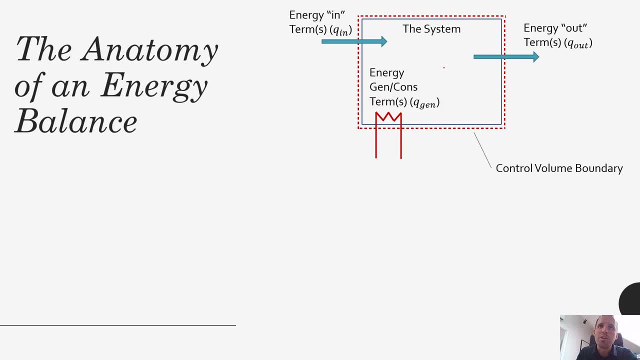 So we're talking here about thermal energy. So we talked about energy. You can't create it or destroy it, but you can convert it from one form to another. So a generation term could be something like electric generation. So maybe if we're doing a thermal energy balance, 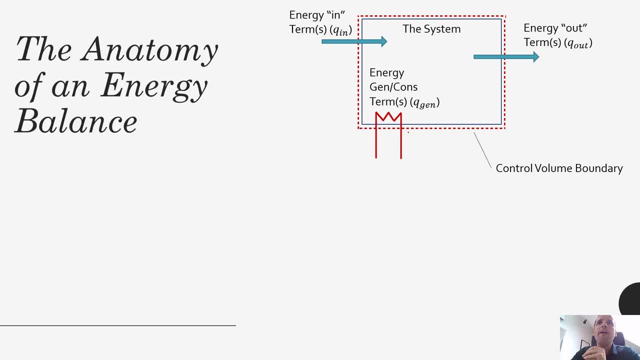 and we have this electrical resistance heater in our system. well, really, what's happening is we're converting electrical energy to thermal energy, but our energy balance is only thermal energy. So we would treat that conversion of electrical energy to thermal energy, we'd treat that as a generation term in our system. 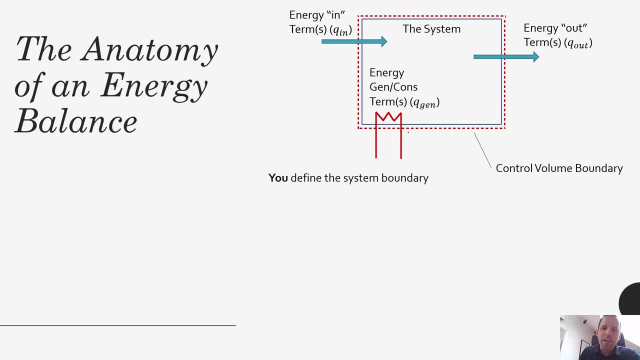 But there would be a number of different ways of dealing with that. So some things to remember. As I pointed out, you're the one that defines the system boundary, and that could be whatever, So you want to make sure that you're defining the system boundary. 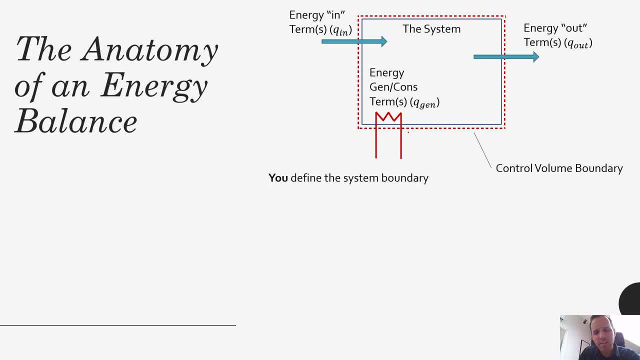 so that you'll create an equation that will be useful, And this is something that I think is just going to take quite a bit of practice. The in and out terms are going to. those are terms that cross the system boundaries. as I mentioned, going in or out. 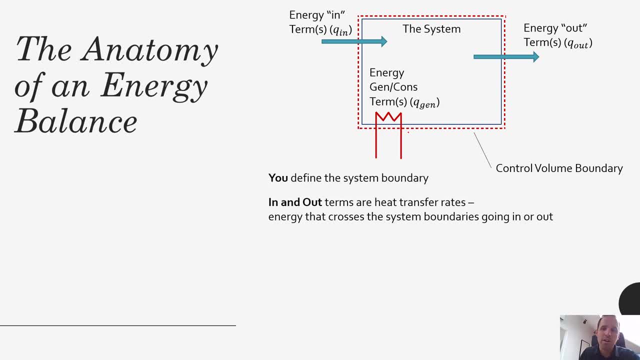 So these are going to come from the three modes, the three different modes of heat transfer: conduction, convection and radiation, And you're going to hear those terms a lot. Definitely commit that to memory. Generation and consumption terms are also rates. 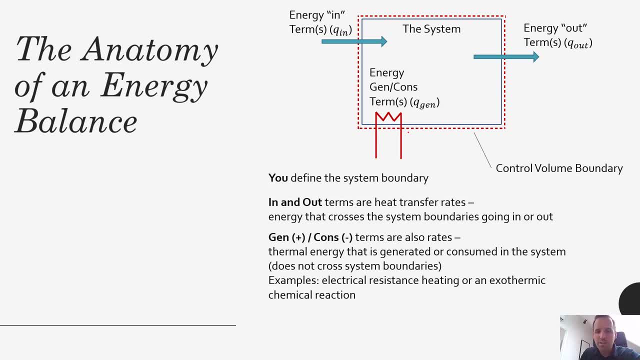 So this is thermal energy that's generated or consumed in the system, and I will typically just use the term generation. A consumption term would just be the additive inverse of a generation term, So examples could be electrical resistance, heating, or this could also be a chemical reaction. 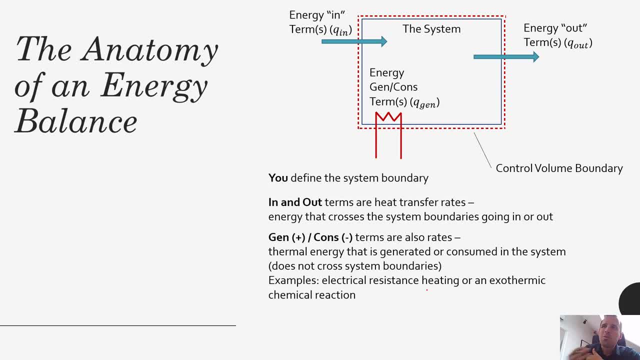 where you're converting chemical energy to thermal energy. So, rather than trying to deal with an energy balance that extends to a different type of energy, like electrical or chemical, we'll just say our energy balance represents thermal energy and we'll treat any conversion of some other form. 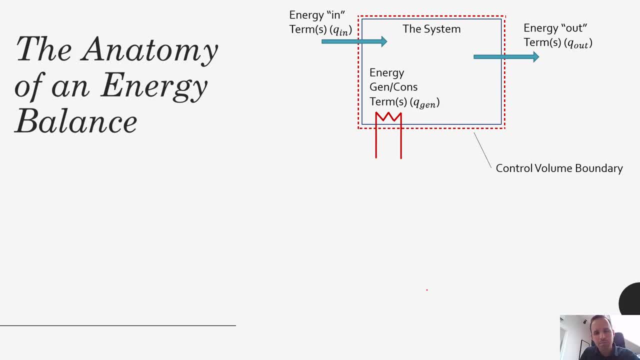 into thermal energy as a generation term. So what are the different terms of an energy balance? So let's put our accounting hats on. So first we want to think about how is energy being accumulated in our system? So we'll have an accumulation term. 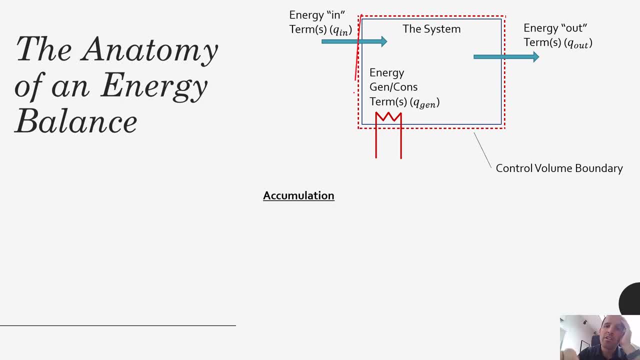 So the accumulation term is going to deal with the total amount of energy in our system. How much is there at any given time? We'll certainly have the in term and the out term and then the generation term. So you'll see this form from me quite a bit. 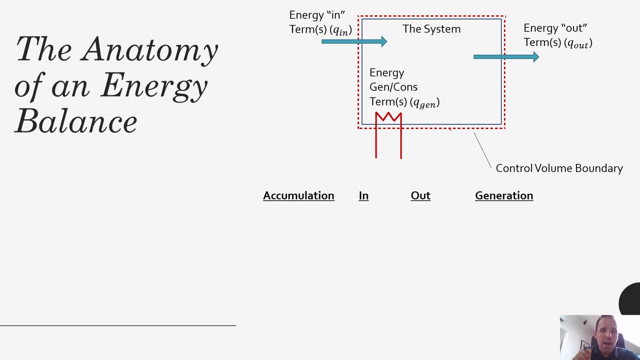 So this is part of our accounting system: How much is being accumulated, how much is coming in and going out, and then how much is being generated or consumed. So in a particular system, your accumulation term might look like this: dE, dt. 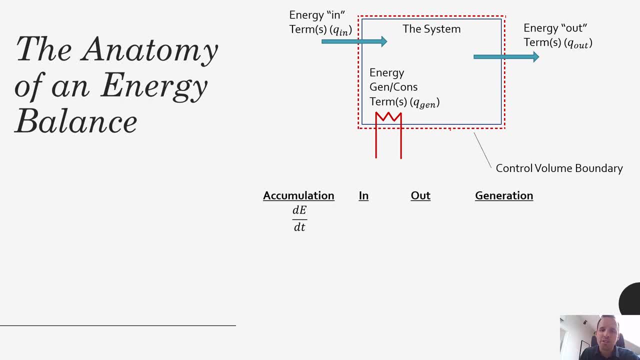 I'm using E to just represent the total amount of thermal energy in our system. That could also be dU, dT, So how much energy total is in our system? How much is coming in? So that would be our in term. 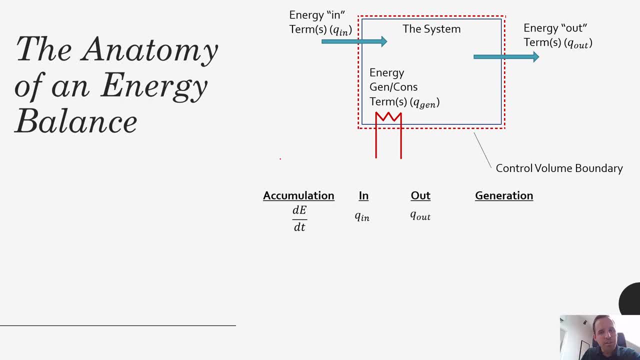 You could have multiple in terms- How much is going out? Similarly, you could have multiple out terms and then generation. So I want you to stop and think. for this particular form of the energy balance, what units should each term have? And if you want to think about this a little bit, 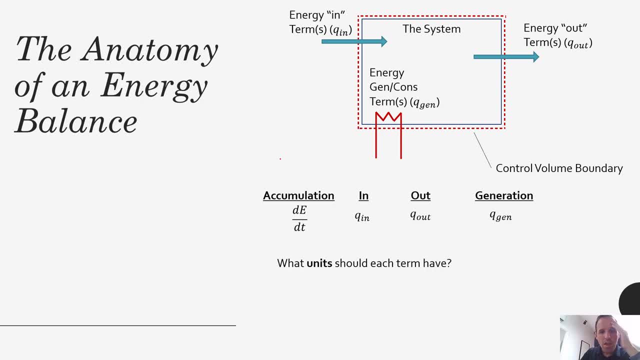 hit the pause button and think about it. All right, so you'll notice that each of these is a rate, a rate of change of energy. So that would have units of watts. So ultimately, we're going to be taking each of these terms and adding and subtracting them. 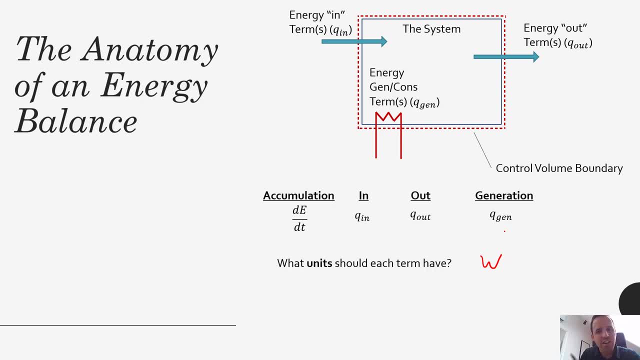 So you can't. it's like an apples and oranges thing: you have to have everything being in the same units if you want to add them together. So this is a very important thing to learn to do as part of your energy accounting system. 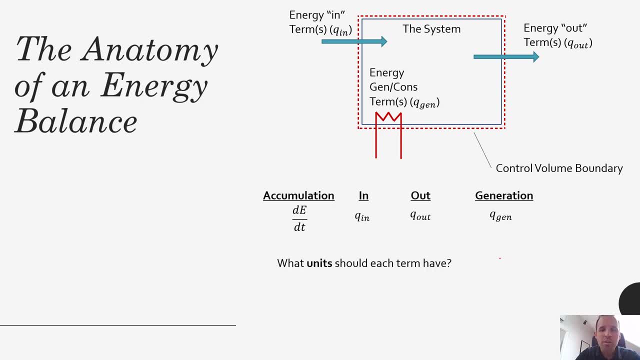 Once you've laid out your terms like this, you're going to want to make sure that each term has the right units. So in the way I've set this up, each of these terms would have units of watts. So again I mentioned this is the rate of change form. 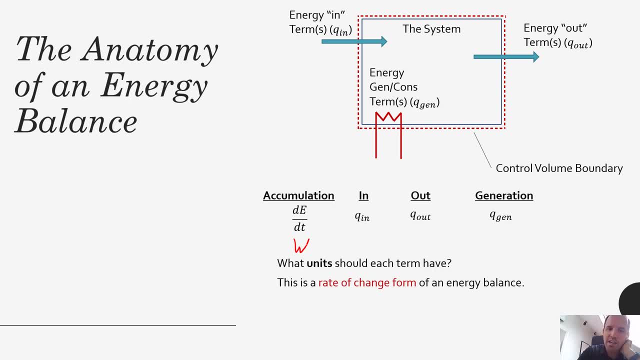 of an energy balance. So we're basically saying how fast is our system accumulating energy, How fast is energy coming in and out and being generated? We definitely want to make sure that those all have units of watts. So the way to set up this energy balance, 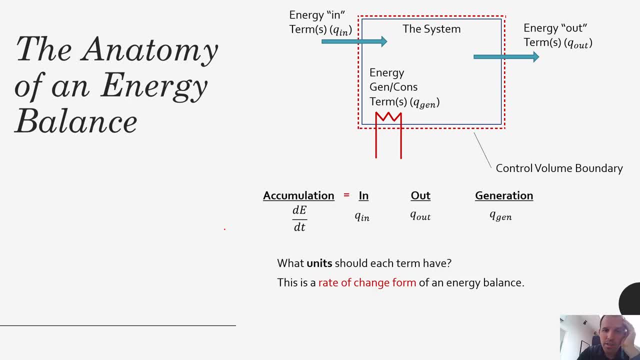 you have accumulation equals. so what's coming in, anything coming in- is going to add to our accumulation term, So we'd expect this in term, to be a positive term, although there may be instances where it's not, and we'll cover those eventually. 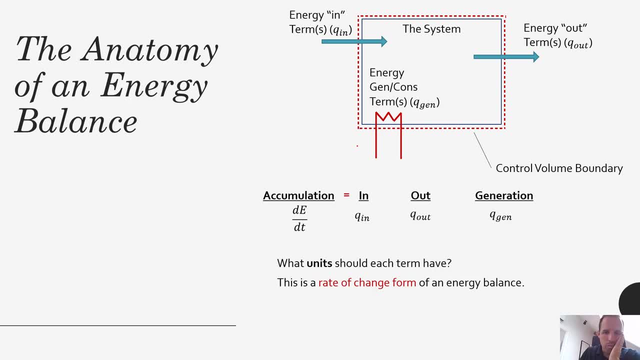 So we have what's coming in minus what's going out, and then we have plus what is being generated in our system, and this will form the basis for our energy balance equation, and it will look something like this: We just take those terms. 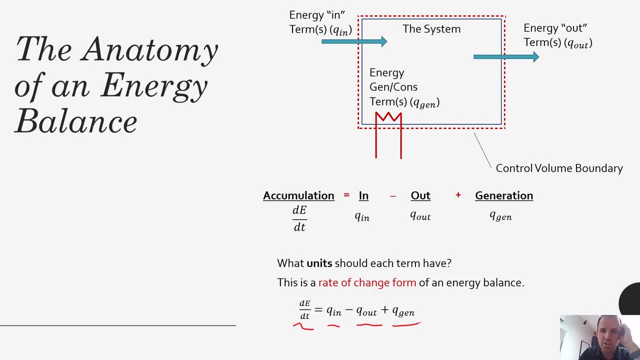 Accumulation equals in, minus, out, plus generation. It will be important to very carefully document how you've set up your rate law, and then you always want to make sure you're subtracting out the out term. So you might set this up so that your out term 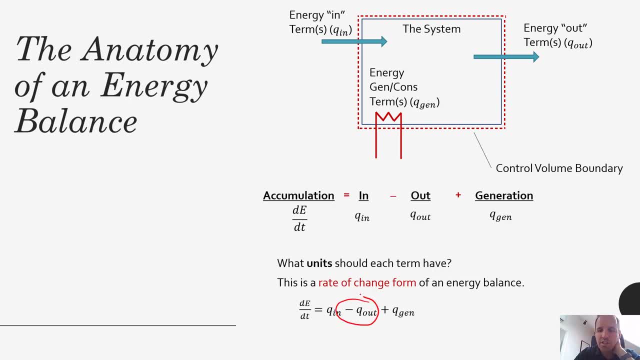 is a positive term, but you're losing that much energy. so when you put it into equation form, you want to make sure you get that minus sign in there. I want to stress: it's very important to make sure that you go through very carefully when you're defining. 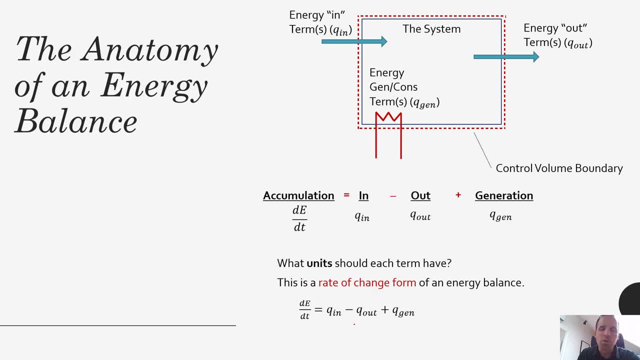 your system boundaries and setting up these rates, that you have a really good conceptual grasp of what's happening in your system. If you have that conceptual grasp, it will be much easier to detect when you have some kind of an error in your equation. Okay, so many of the problems we will solve in this class. 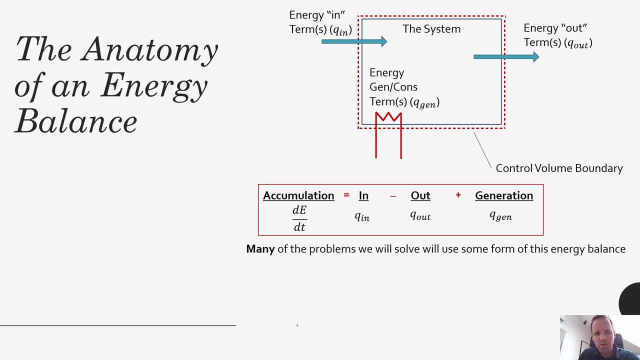 this will be the most common form of an energy balance that we'll use, so that's the one I'm showing you here. is this rate of change form? The problems that there will be, problems that we solve that don't necessarily require an energy balance. 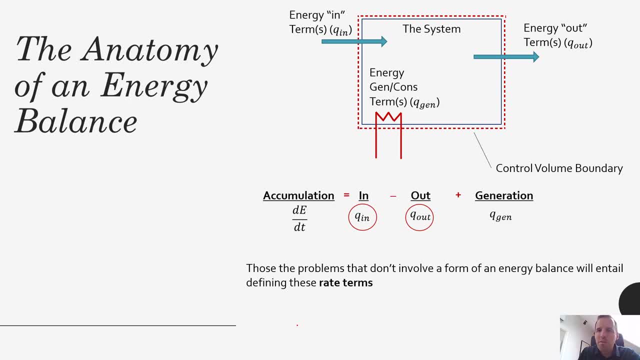 I would call these rate problems. So sometimes there may be a problem that will just ask you how fast is energy leaving, or how fast is it coming in, or how fast is it being generated. In that case we'll use those laws of heat transfer. 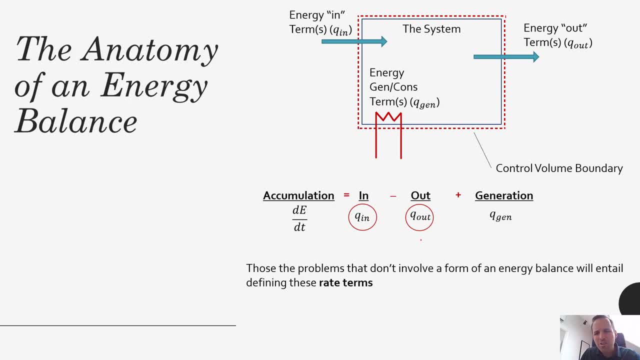 to figure out the in and the out terms. Generation term is usually a little bit simpler, So there may be some problems that are just what's the rate and we'll just use that rate. These rate equations are going to come from the three different modes of heat transfer. 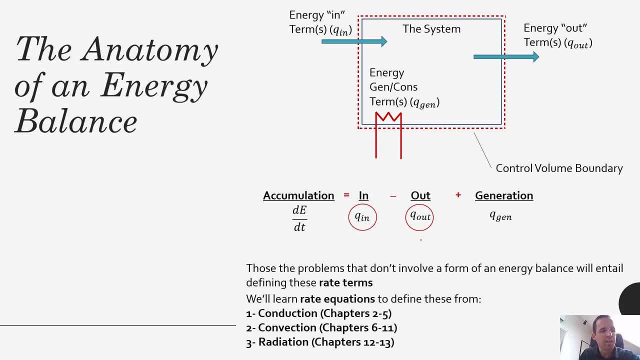 conduction, convection and radiation, And in the next few lectures we'll teach, we'll introduce these different forms in more detail and start talking about the rate laws or the equations that are going to tell us how fast energy is coming in or out. 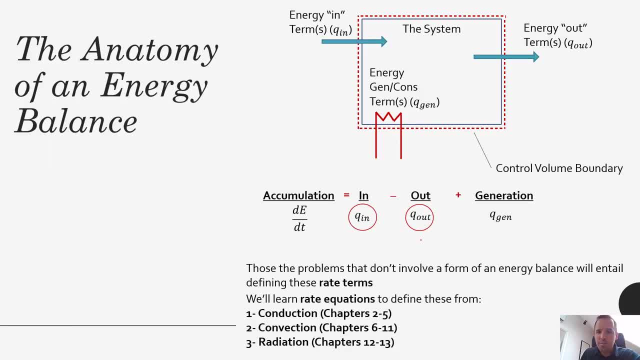 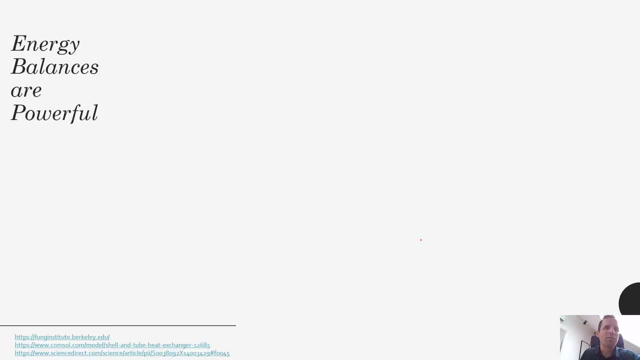 While this sounds really simple, this looks like a really simple system and I hope you're all staying with me. you can expand this system to become something much more powerful. So you're going to take those accounting skills and your very simple and clear system. 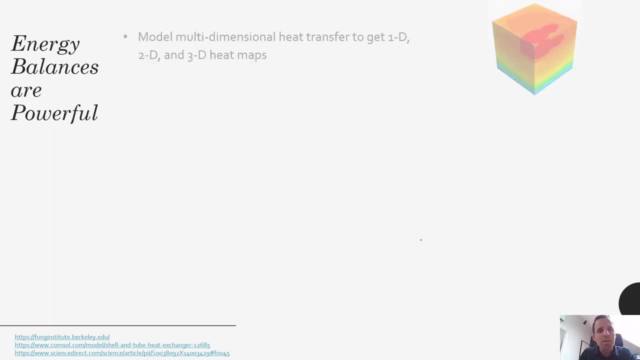 and you can expand that to be to cover thousands or millions of different energy balances. So this could be used to do to generate one-dimensional, two-dimensional or three-dimensional heat maps. So this picture here is a three-dimensional heat map. 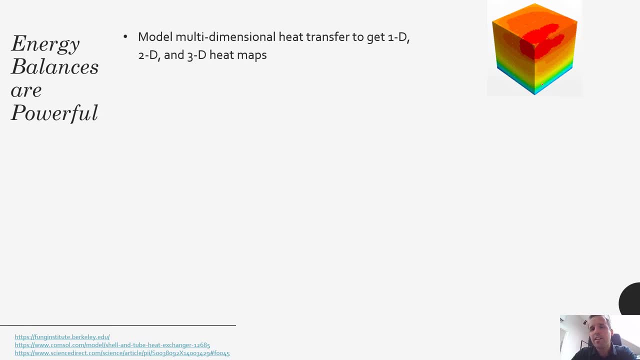 And the way that you would solve a system like this is to take that big chunk of material and divide it up to thousands or even millions of different tiny little control volumes. Each one of those control volumes is going to be coupled with an energy balance equation. 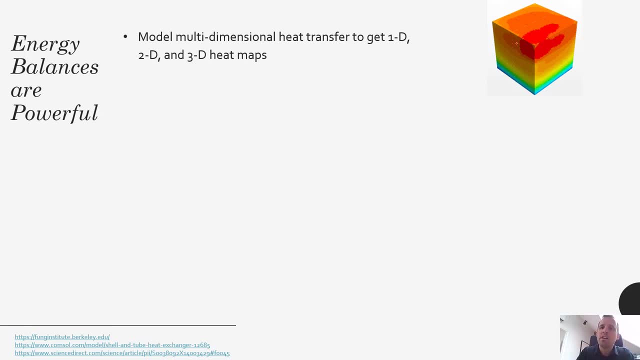 and then by solving all of those equations simultaneously, you can get this really detailed and complex heat map. You can do this same kind of thing to do something like model a heat exchanger. We're going to cover heat exchangers in Chapter 11.. 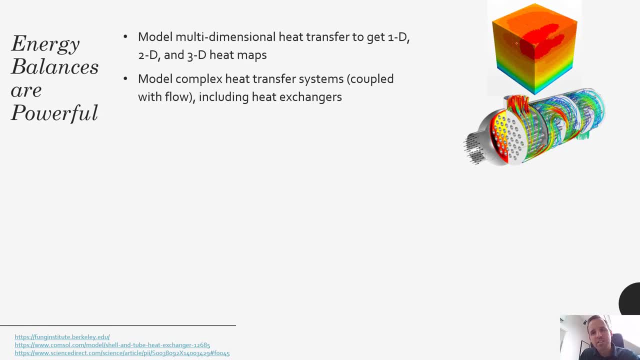 But you can use very sophisticated software to give you changes in temperature in addition to flow, which is where fluid mechanics would come in, to come up with very complex models to understand how your design might perform. or you could use this to detect where something is going wrong in your system. 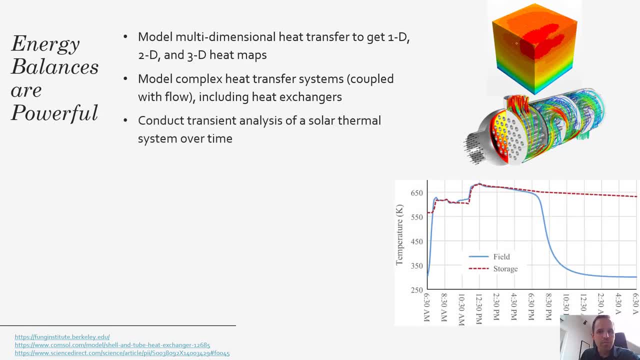 You can also add in transient analysis So you can model very complex systems like a solar thermal power plant and capture how a bunch of different components of that plant are changing over time. So I really want to emphasize that, while I tried to present a very, very simple energy balance, 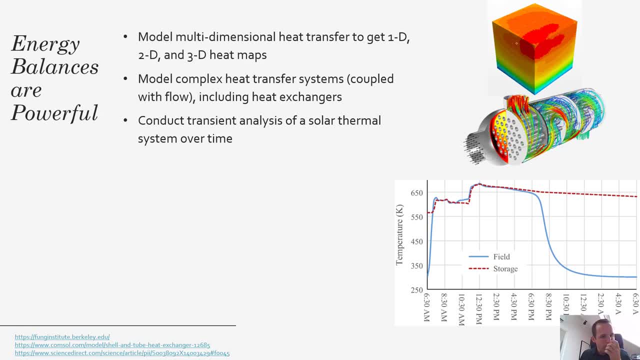 in the last few slides. you can take that same concept and really, without adding too much complexity, you can model amazingly complex systems and actually these can become really fun problems to solve. So tips for being a good energy accountant: Take the time to really digest the concepts. 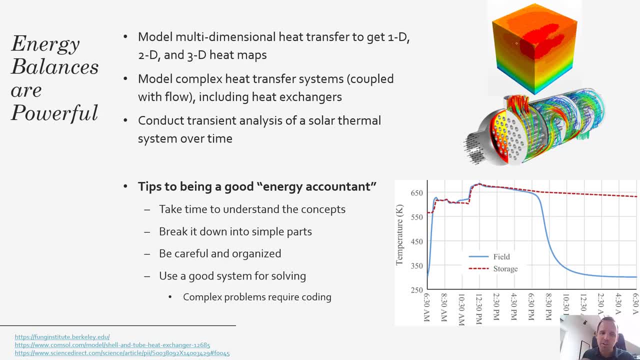 Take the time to set up your system boundaries, to identify the Q in and Q out terms, the generation terms and the accumulation terms. So if you're doing that, you're already breaking that down into very simple parts. You're taking something that could be complex. 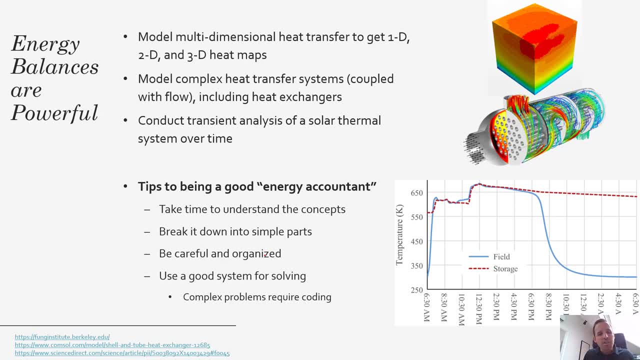 and learning to break it down into really simple pieces and then you can use something like computer software to solve a very complex system like those that you're seeing here on the right. So be very careful and very organized and if you set this up well, 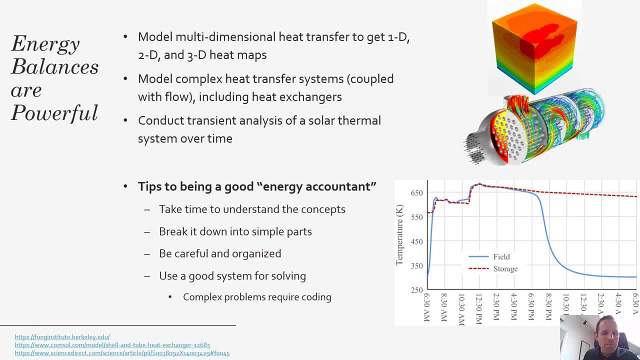 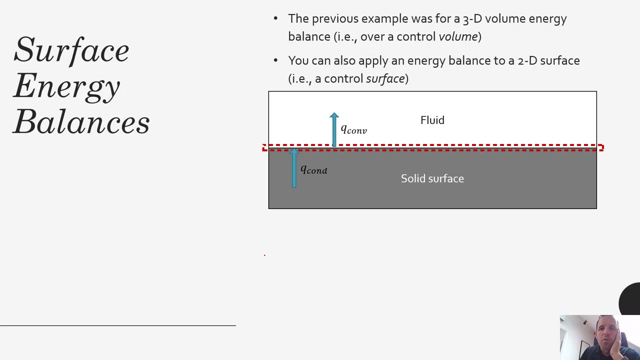 and are very systematic about it, then you can take very complex problems and plug that into a system like computer software to solve a much more complex problem. So I mentioned the energy balance. we did before was for a control volume. We thought about our space or that matter. 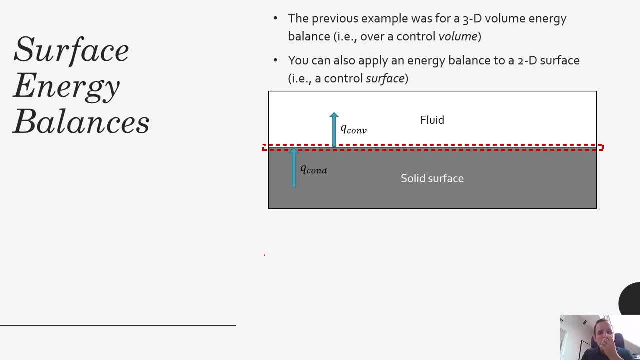 as a three-dimensional object. Well, you could also do this on a two-dimensional object. so by doing a surface energy balance. So let's say that we have a wall system here- You'll learn later this is called a plane wall- and we have this solid surface bumping up against this fluid. 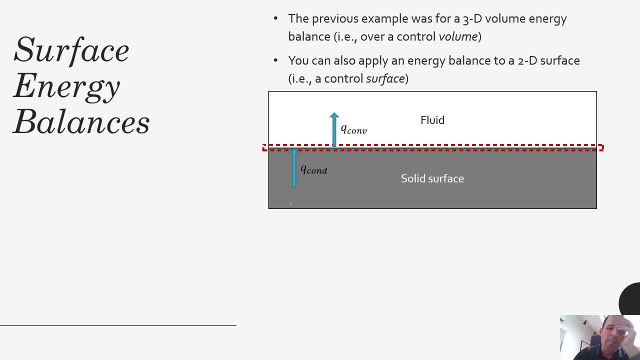 So we're going to have conduction heat flowing through our solid. We'll learn about these different modes soon. So we'll have conduction coming in and convection leaving. So it may be useful for us to just look at this plane here. 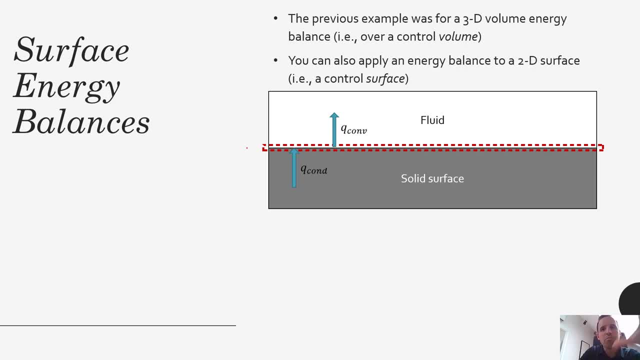 and this would basically be just a planar system. It has no volume where energy could come in and go out. These will be another form of energy balance that could be really useful to us. So if we use that basic form, accumulation equals in minus out. 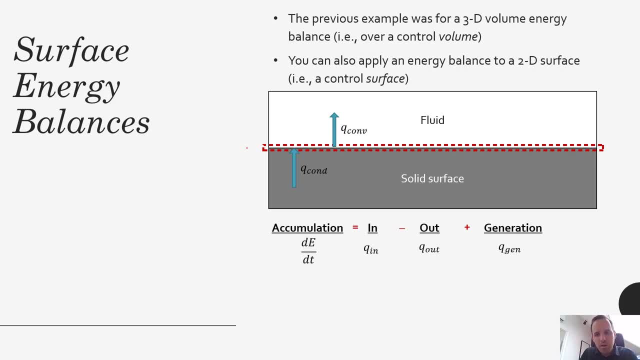 generation. Let's just look at our different terms. So here are the same terms. I'm keeping this really simple. We're going to go through later and quantify these terms in more detail. Our accumulation term would be zero for a surface energy balance. 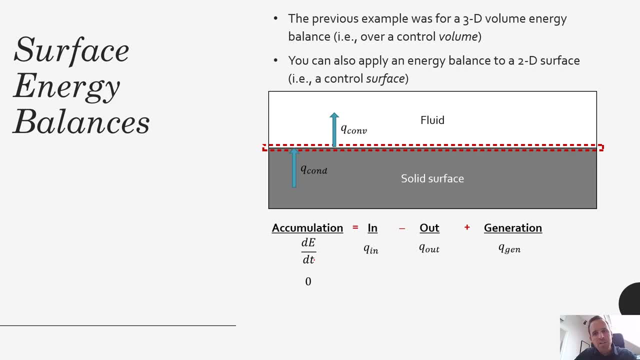 and that is because it's just a two-dimensional system. It has no volume, It can't accumulate anything because it has no really physical space to accumulate something. It's just a two-dimensional plane. It could certainly still have an interim In this case. I've specified that interim. 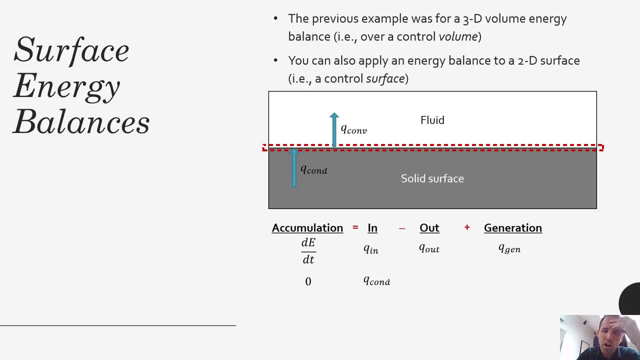 is coming in by conduction. so I'm using q subscript cond or q by conduction coming into my system, And then I would have q leaving my system by convection. And if you don't know what those terms mean yet, don't worry. 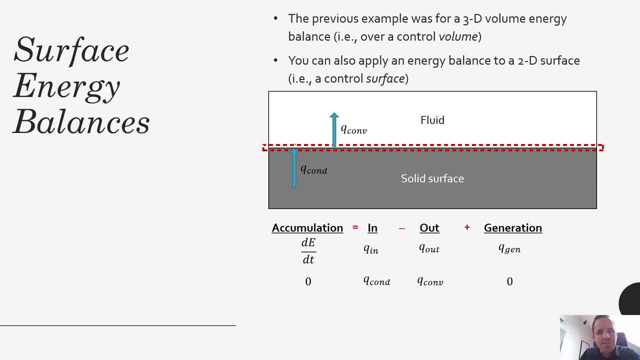 We're going to cover them in the next lectures. This system would also have zero generation, At least in this course we're going to mostly be dealing with volumetric generation terms. So if our system has no volume, it will not be able to generate energy. 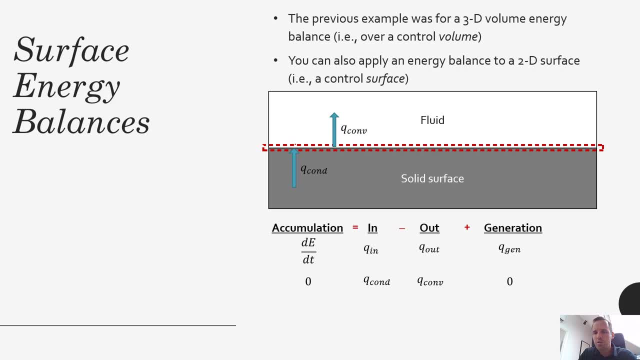 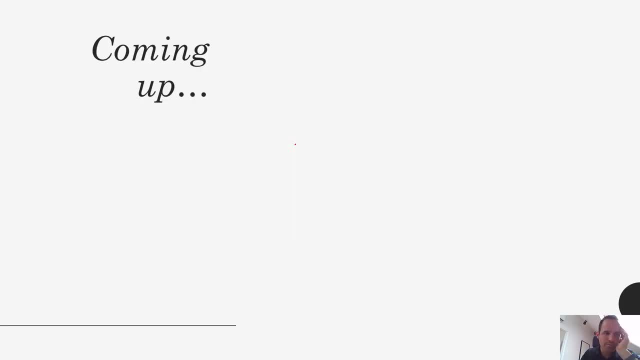 If there's no physical, actual space to deal with, because it's only two-dimensional and flat, then there would be no room to have generation. But certainly there may be other ways of thinking about that. Alright, so coming up, we are going to learn how to quantify. 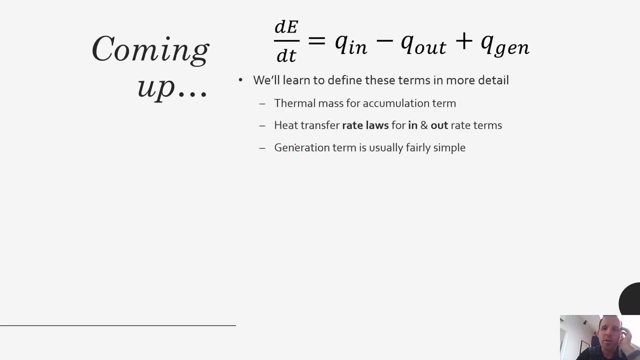 each of these terms in more detail. So the thermal mass we'll use for the accumulation term. that's going to have terms units of density, of heat capacity and of change in temperature with time. We're going to use these heat transfer rate laws. 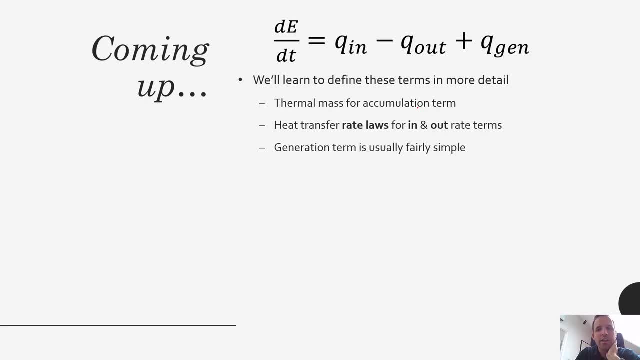 which I'll introduce in the next lectures to quantify our in and out terms. And then the generation term, as I've mentioned, is usually fairly simple. the way we'll deal with it: There will usually be some kind of mathematical equation to plug in there. 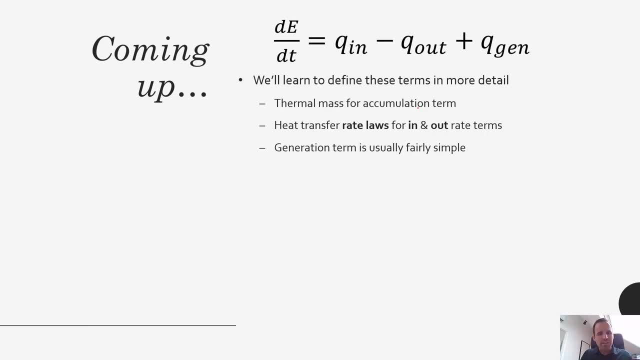 So we've learned how to do an energy balance, or at least how to start thinking about an energy balance. So what heat transfer is going to teach us really well is: how do we document these different flow of heat terms? I have tried to put this energy balance. 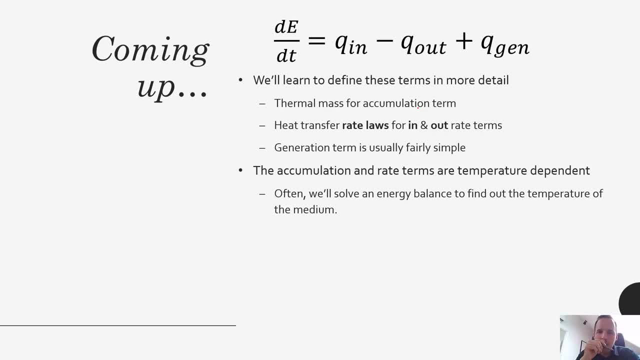 into terms that are very simplistic. So just a single algebraic formula. this does look very simple, But eventually we're going to put in terms where each of these are temperature dependent. We'll have more algebra and calculus going into each of these terms.